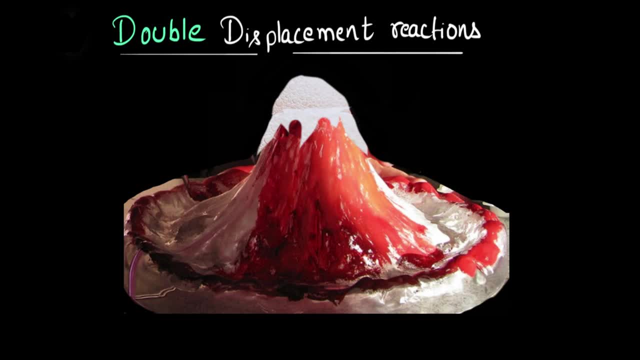 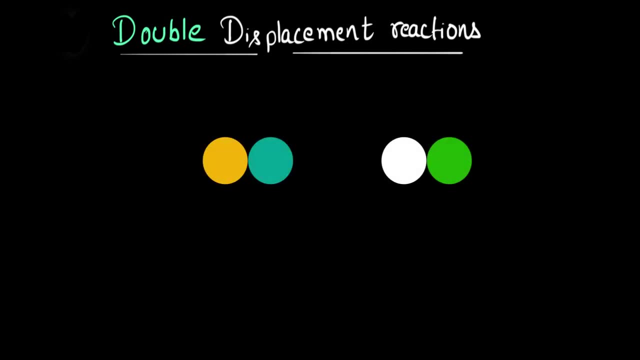 I will also show you by making one volcano. So let's begin. So if I have to explain you in short, in double displacement reactions the ions of the reactant, they exchange position, Something like this. Now let's see how to write this in a chemical equation. 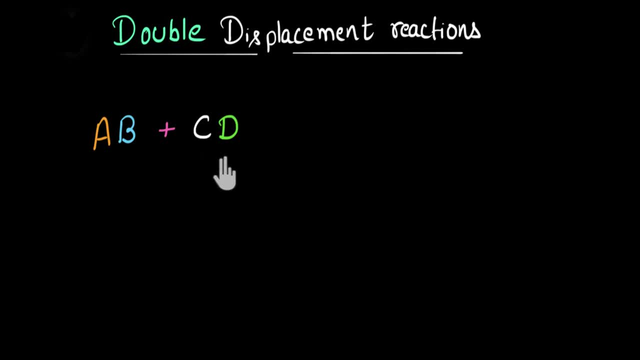 So here I have two random reactants, AB and CD. Now if double displacement reaction is happening here, then the ions are going to exchange position. So here in this reaction, A will go and displace C and form AD, whereas C will go and displace A in turn. 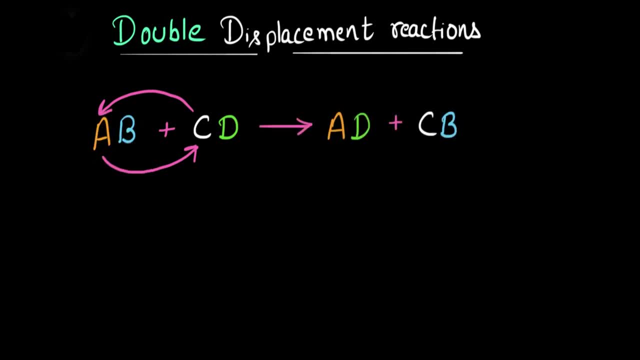 and form CB And finally our products are going to be AD and CB. Now you can see that. why this is called a double displacement reaction? because in a way, we can see that A is displacing C and C is in turn displacing A. 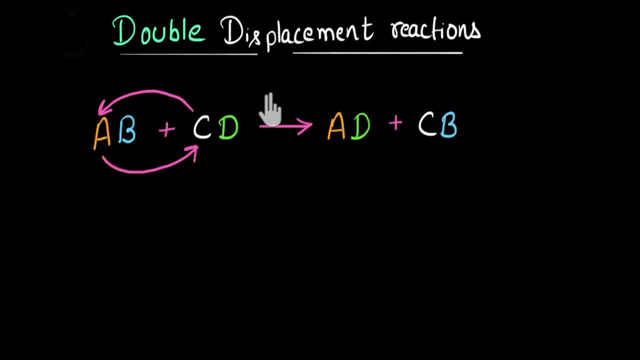 And since there are two displacement, so we can call it a double displacement reaction. Okay, now let's look at an actual reaction. So here I have hydrogen chloride and sodium hydroxide, And when they react it is going to be a double displacement reaction. 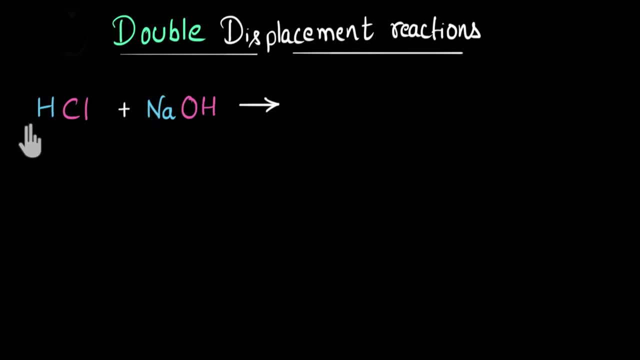 meaning the ions are going to exchange position here. So here hydrogen ion is going to exchange position with basketball, exchange position with sodium ion. let's say So here hydrogen will displace or take the position of sodium and form HOH, or I can say H2O, right. 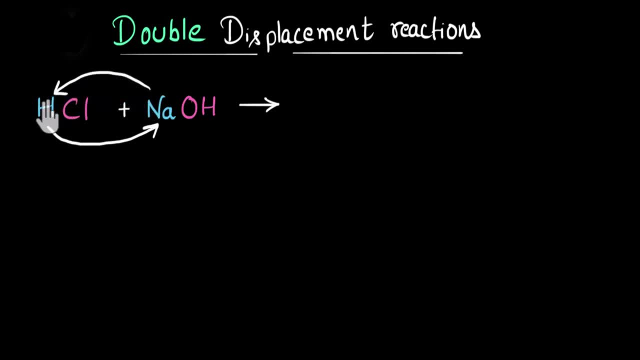 Which is water And sodium, will in turn take the position, displace hydrogen and form sodium chloride, NaCl, And this is going to be our product: HOH or H2O and sodium chloride. Now I've got two reactions. 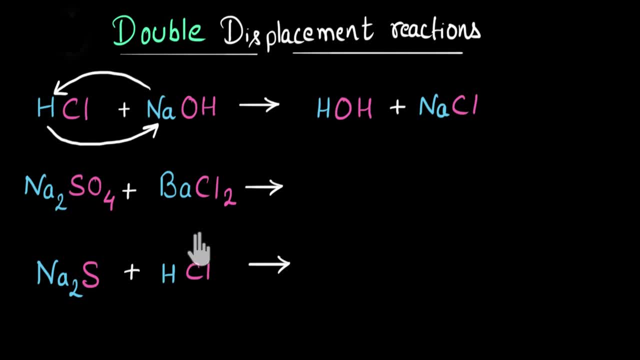 and both of these are double displacement reactions. Now I want you to pause the video and try to find out the product of these by yourself first. Now, if you have tried it, let's see So here in this reaction, since this is double displacement. 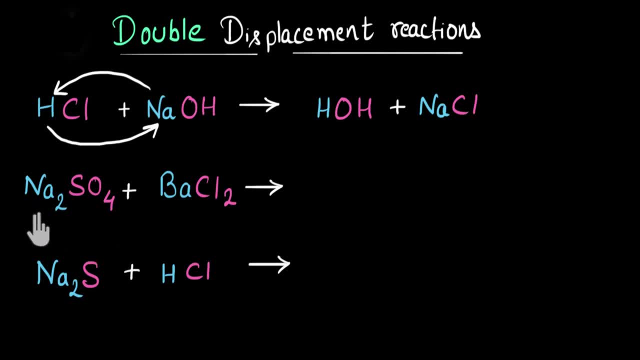 ions are going to exchange position Here. sodium will exchange position with barium. So okay, sodium displaces barium in one sense and forms sodium chloride, And in turn, barium takes the place of sodium and forms barium sulfate. 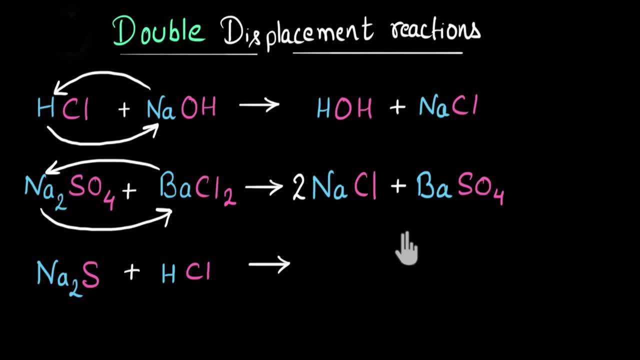 So the product is going to be sodium chloride and barium sulfate. Now let's look at this reaction. So here also double displacement, so ions exchange. So sodium takes in the place of hydrogen and forms sodium chloride, And hydrogen in turn takes the place of sodium. 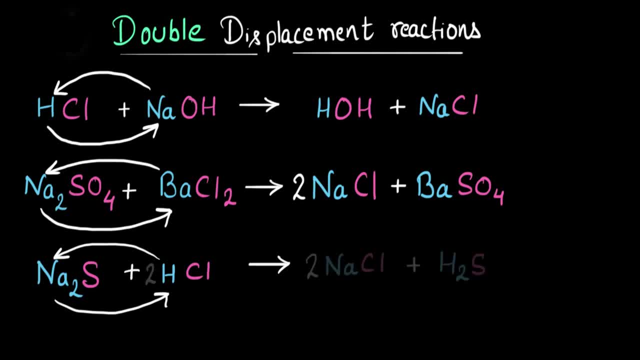 and forms hydrogen sulfide. So the product is going to be sodium chloride and hydrogen sulfide. So okay, with this you understand the basic structure of double displacement reactions. But you might be having many questions like over here: why sodium chloride and hydrogen sulfide? 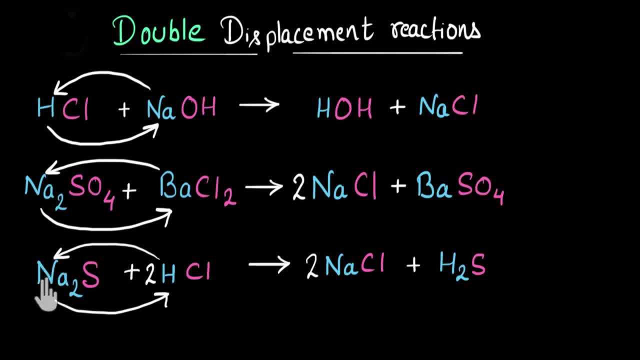 Why is sodium only exchanging position with hydrogen? Why can't it exchange position with, let's say, chlorine? Or can sulfur exchange position with chlorine? Or what is happening at the core, Like, how are these reactions even taking place? Now, all of these questions are amazing questions. 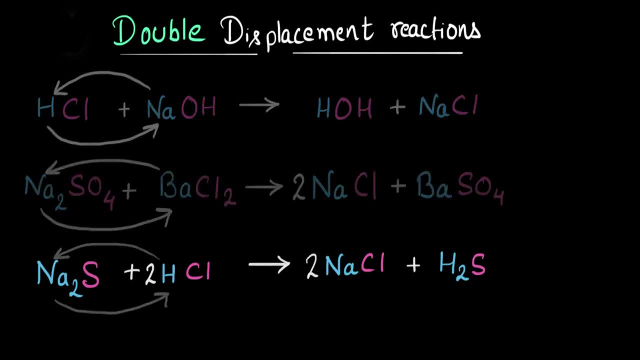 But to understand these, let's look at a little bit in detail. So here I have sodium sulfide Na2S. Now if I put this in water- meaning I'm taking an aqueous solution of sodium sulfide- then in that case this molecule is going to disperse. 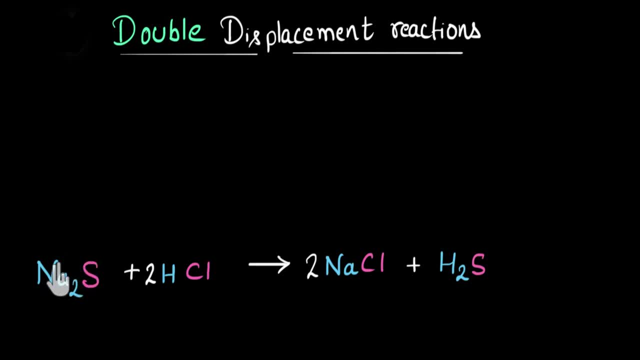 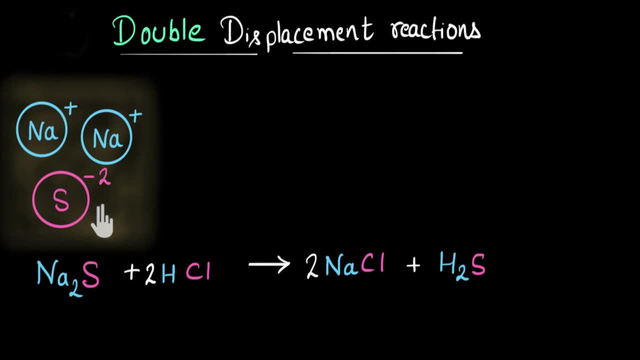 Dissociate or break down into its ions. I will get sodium ion and sulfur ion, Something like this. Here I'll get sodium ion and sulfur minus two ion. Now this is nothing to be worried about. Many molecules when put in water. 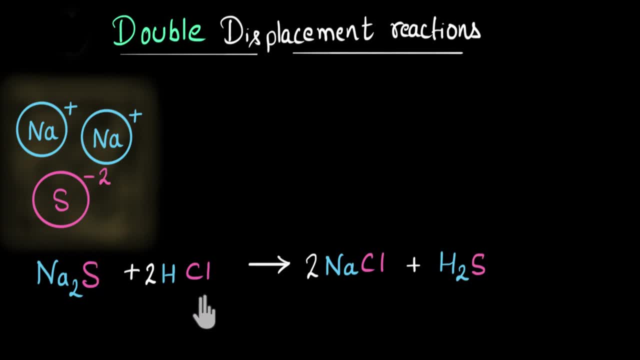 they will dissociate into its ions. Similarly, over here, HCl, when put in water, This will also dissociate into hydrogen ion and chlorine ion. Now see why certain molecules dissociate in water is something that we will talk about in a separate video. 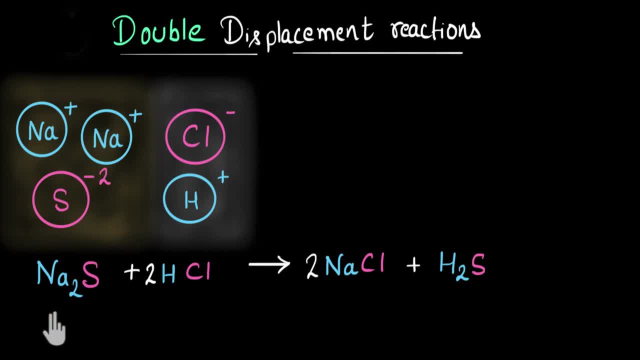 So if I only have a solution of sodium sulfide, then in that case I will only have sodium plus ions and sulfur minus two ions, And they will be attracting each other, Because we know that opposite charges: they attract each other. 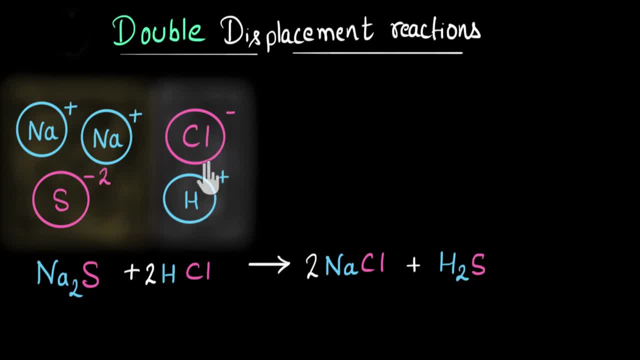 But if to that solution I also add a solution of HCl, meaning now I also have H plus ions and chlorine minus ions? Now see, sodium has no reason just to be attracted towards sulfur. Now it also sees that there is chlorine minus ions. 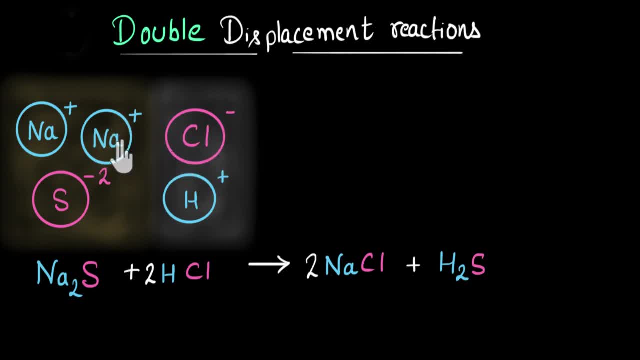 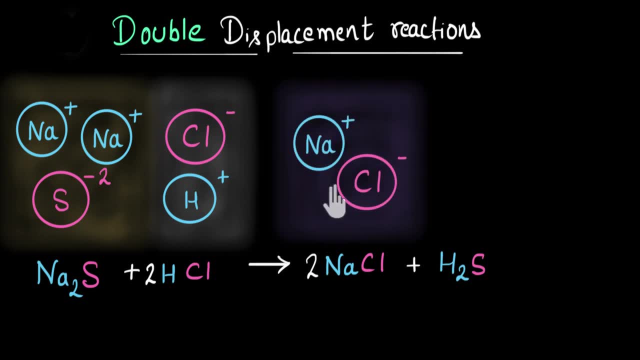 Now it also sees that there is chlorine minus ions. Now it also sees that there is chlorine minus ions. So some of sodium will also get attracted to chlorine minus ion And we will have sodium chloride being formed, Which will look something like this sodium chloride. 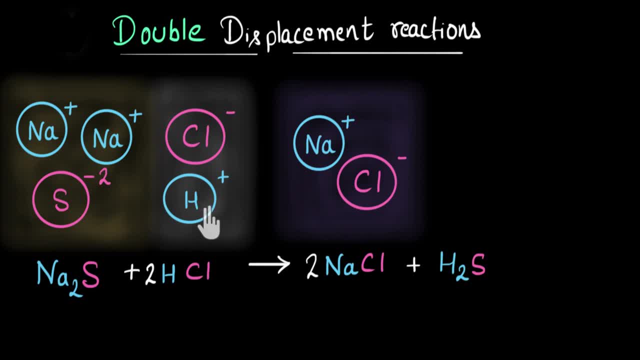 And similarly over here. hydrogen that was earlier only attracted to chlorine now sees that. okay, there is sulfur minus two ions also present in solution. So some of the hydrogen ions. they will get attracted to sulfur minus two ions And they will form hydrogen sulfide. 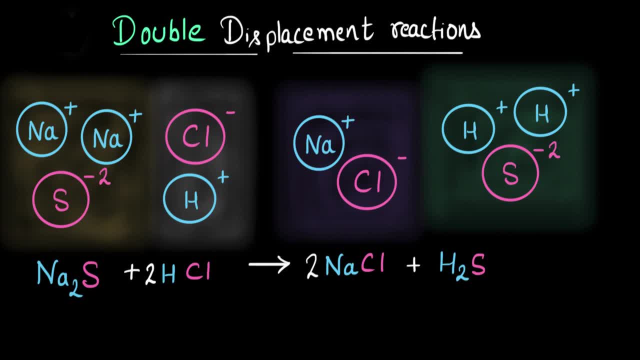 Something like this. Now, this is something that is happening in every double displacement reaction: First of all, the reactants will break down into their ions, and then the ions will exchange position to form new, new products. Now this model can help us answer all our questions. 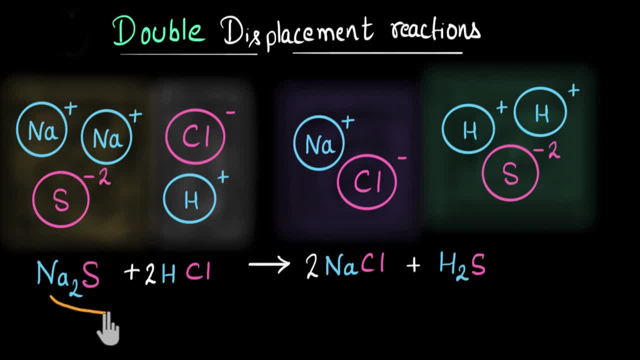 So the first question is: can sodium exchange its position with chlorine instead of hydrogen? I want you to pause the video and think about this by yourself first. Now, if you have tried, let's see. So see if sodium exchanges position with chlorine. 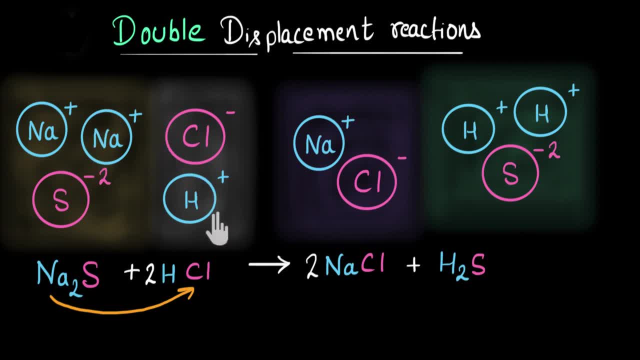 that means that a molecule of sodium and hydrogen should be formed right. But see sodium and hydrogen. both are positively charged And we know that. like charges, they do not attract but they repel each other. And if they're repelling, 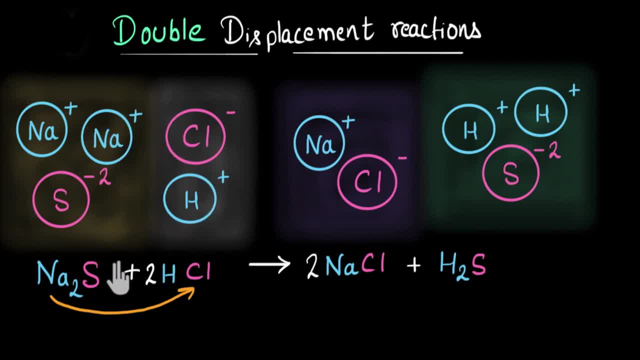 there's no way that they can form a molecule right? So that's why sodium cannot exchange position with chlorine. In fact, no positive ion can exchange position with a negative ion. Positive ion can only exchange position with another positive ion. Now another question is: 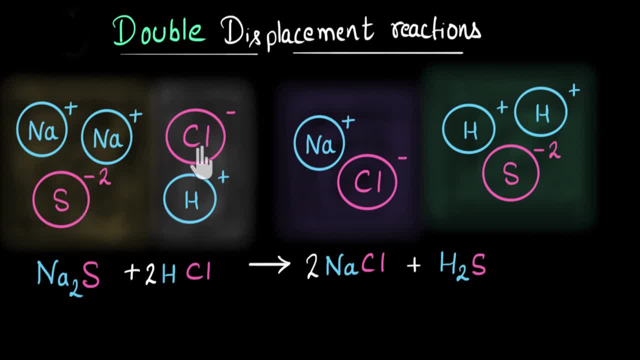 can sulfur exchange position with chlorine? So yes, that is definitely possible. See, if sulfur comes here instead of chlorine, it will form a molecule with hydrogen, hydrogen sulfide. And that is what we are actually getting over here: hydrogen sulfide. 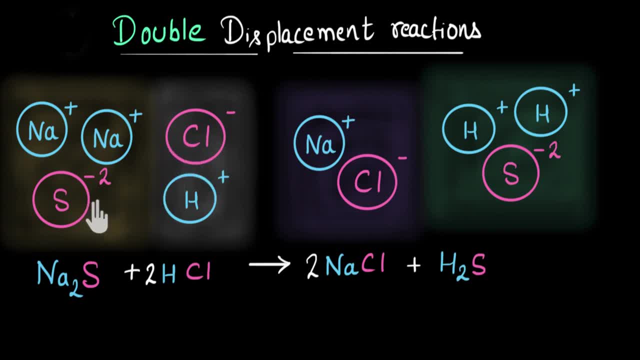 Similarly, if chlorine exchanges position with sulfur, it will have to form a molecule with sodium and we'll get sodium chloride. And that's what we are getting over here, right. So that's what happens in double displacement: Either the positively charged ions 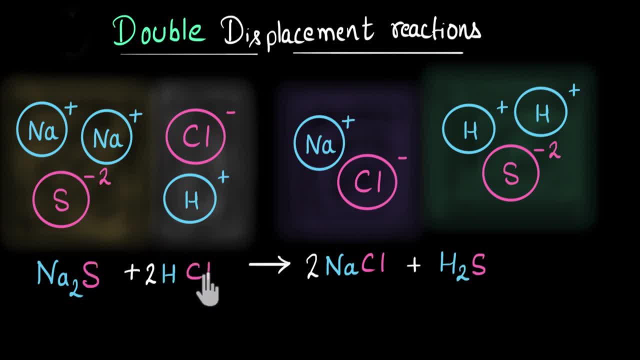 they exchange position, or the negatively charged ions they exchange position? They both basically mean the same thing, As long as you do not exchange position between a positively charged ion and a negatively charged ion. Now there is one more question to answer. You might be wondering, Ram, when we mix the reactants. 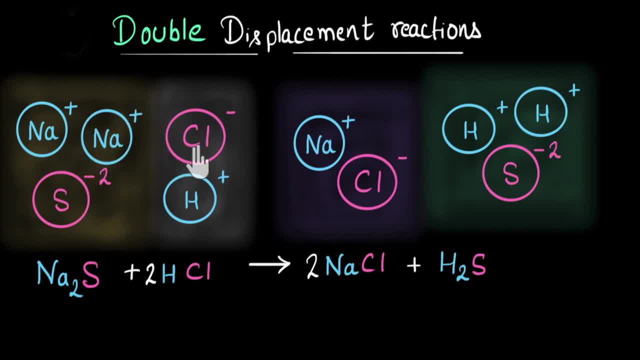 some of the sodium ions. they got attracted to chlorine ions And that's how sodium chloride was formed And we wrote that on the product side. But rest of the sodium was still attracted to sulfur, right, And we should still have some sodium sulfide ions. 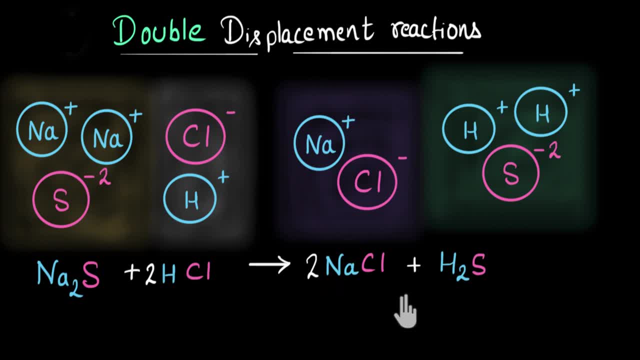 And we should also write that on the product side. Why aren't we mentioning that? Similarly, some of the hydrogen ions. they were attracted to sulfur ions And we got hydrogen sulfide And we wrote that on the product side, Whereas rest of the hydrogen 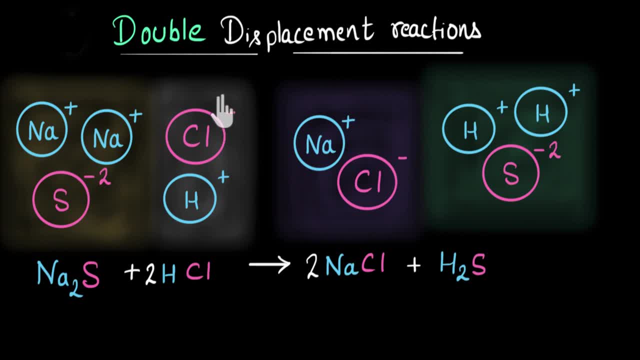 should still be with chlorine right, And we should still have some hydrogen chloride left, And we should also write that on the product side. Why aren't we writing that? So that's a very good question, see hydrogen sulfide. this is here a practically irregular process. 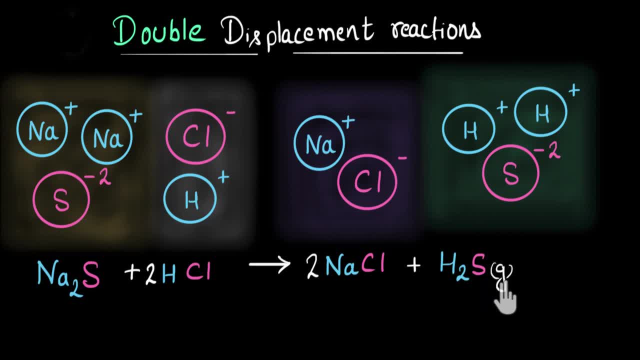 But you can bemark it. This is a gas and this cannot be present in a liquid. This will escape out of the liquid. What this means is the moment hydrogen ions and sulfur ions- they come close together and combine, they will form hydrogen sulfide, which is a gas. 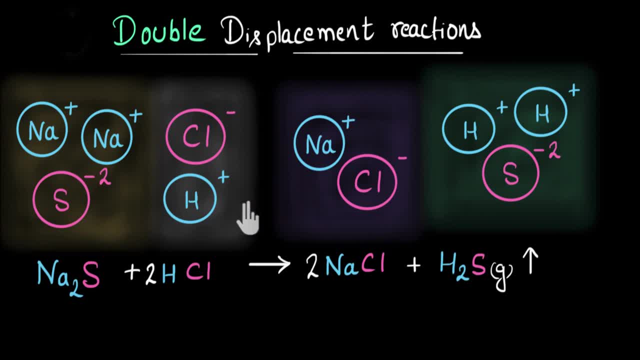 and this gas will escape out of the solution. Now, what this means is, as time passes by, more and more hydrogen ions and sulfur ions are getting lost out of the solution, So we are no longer having sulfur ions in the solution. That means we can no longer form sodium sulfide. 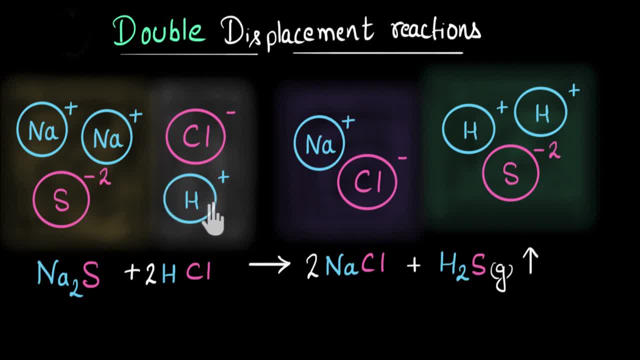 And also we are no longer having hydrogen ions in the solution and that means we can no longer form hydrogen chloride, The hydrogen and the sulfide ions. they will combine together to form hydrogen sulfide gas, which will escape out of the solution. And similarly, if we take this example, 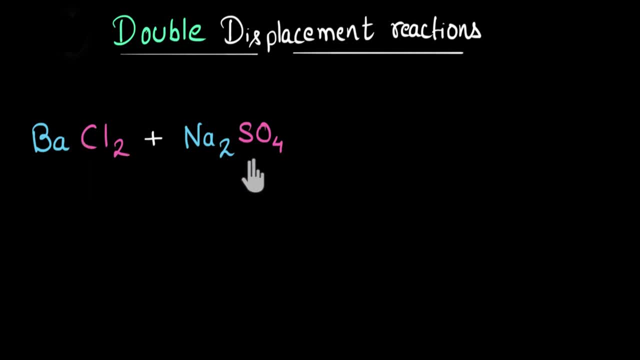 barium chloride plus sodium sulfate. Now this is also a double displacement reaction. When we mix these in an aqua solution, or that means in water, then barium chloride. this will dissociate into its ions and its ions are going to be barium plus two ions. 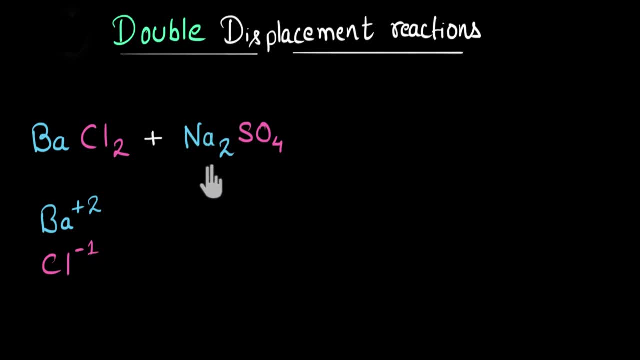 and chlorine minus one ion. Similarly, sodium sulfate. this will also dissociate into its ion sodium and sulfate ion, Na plus one and SO four minus two. Now see now barium plus two ion. this can get attracted to even sulfate ion. now 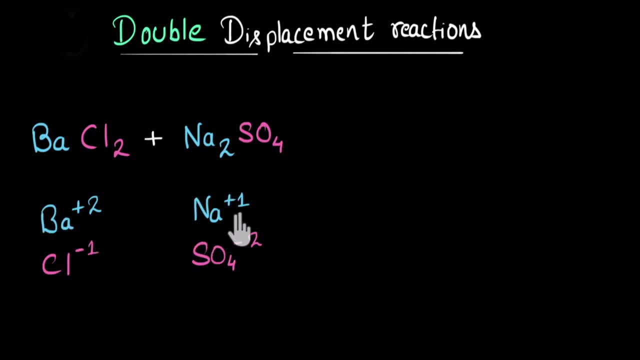 and this will form barium sulfate, also, Similarly, sodium ion. now this can get attracted to chlorine ion also and this will form sodium chloride, And so the products are gonna be barium, sulfate and sodium chloride. Now- see the moment, barium ion and sulfate ion. 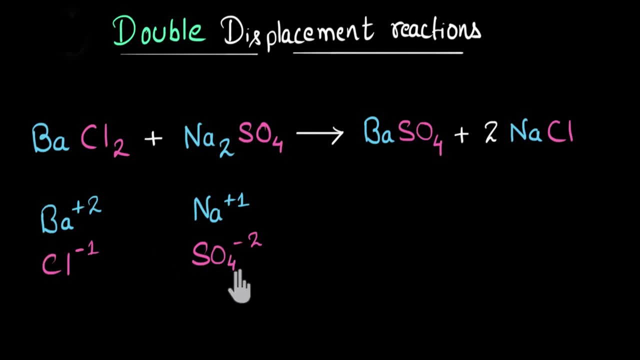 come together they form barium sulfate, which is insoluble in water Meaning. it will settle down out of the solution. It will precipitate out of the solution, Just like when you mix sand in water. the sand, after some time it settles down right. 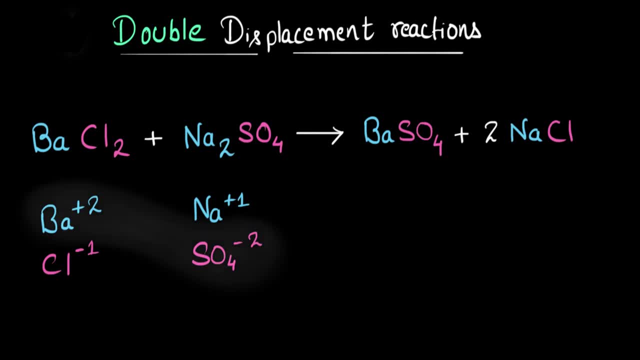 Something very similar is going to happen with barium sulfate. That means, after some time, barium and sulfate ions- they won't be available in the solution anymore. The only ions available in the solution are of sodium and chloride, which will form sodium chloride. 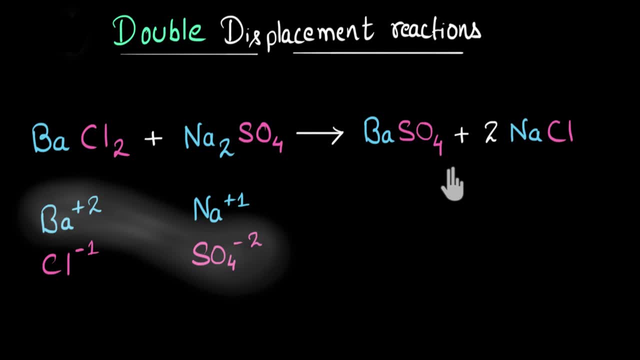 and barium sulfate will settle out of the solution And since we don't have any barium ion left, we can't have any barium chloride being formed. And similarly, since we don't have any sulfate ion left, we can't have any sodium sulfate being formed. 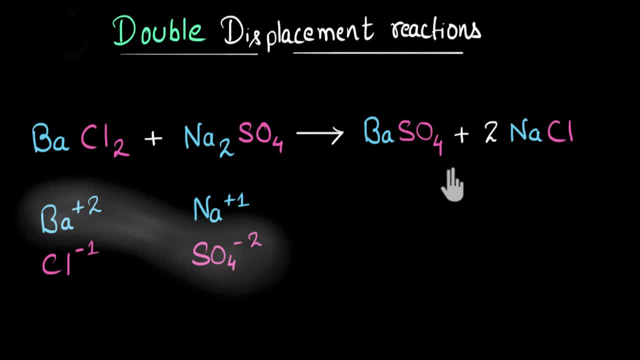 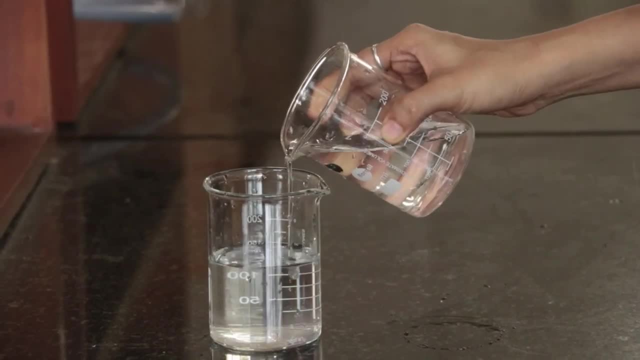 So just two products Here. I have an experiment to show the same thing Here. I've taken barium chloride solution and sodium sulfate solution, both of which are colorless, But the moment I mix them I am getting a white compound being formed. 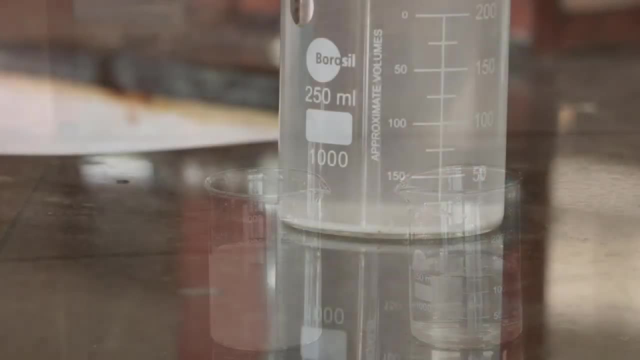 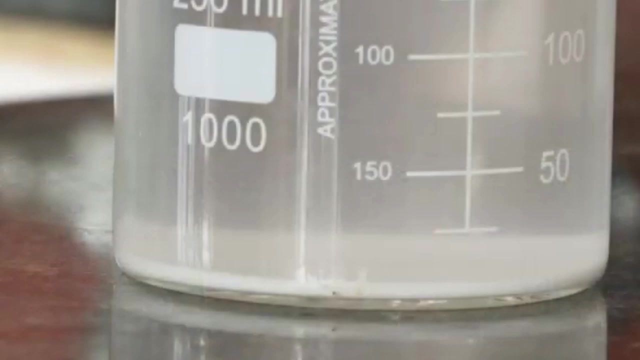 Now that is barium sulfate, And after some time this barium sulfate is going to settle down at the bottom of the flask. Now, such reactions in which a precipitate is formed, something that settles down, these reactions are also called as precipitation reactions. 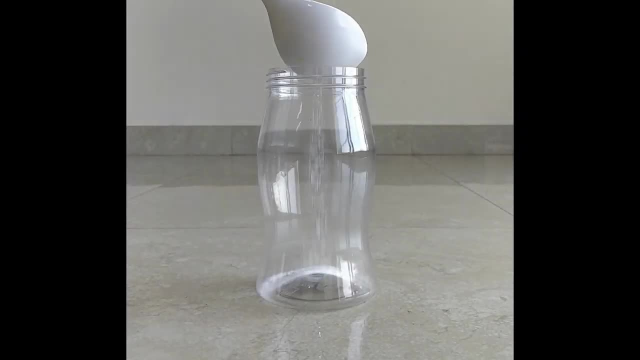 Now let's make our volcano. For this, you'll require baking soda and vinegar. Now, the moment you add vinegar to baking soda, wow, you can see the amount of froth being generated. A lot of gas is evolving over here, And if you put this reaction in a small volcano, 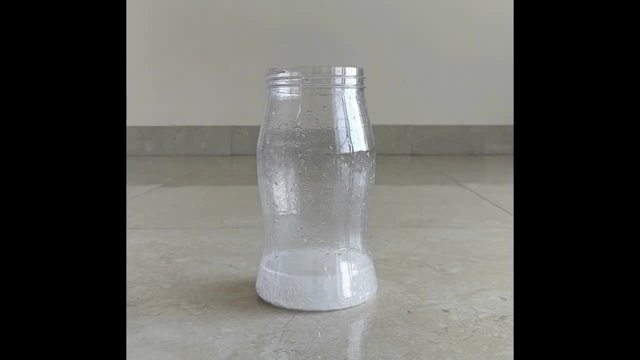 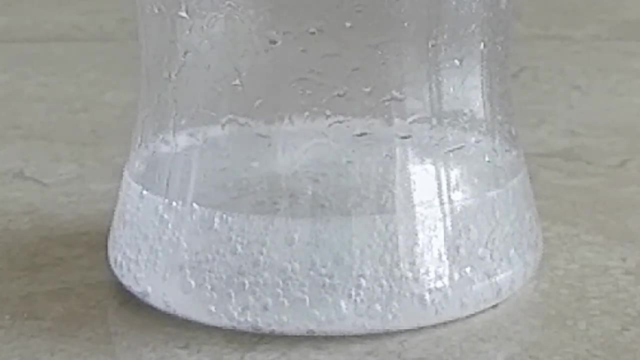 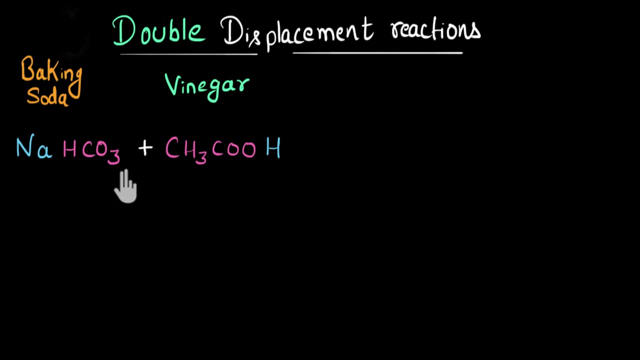 you will have a lot of bubbles coming up And this will look amazing. In fact, if I zoom in, you can still see the bubbles coming out. Now let's look at the chemical equation of this reaction to understand what's happening. So the chemical formula of baking soda is NaHCO3.